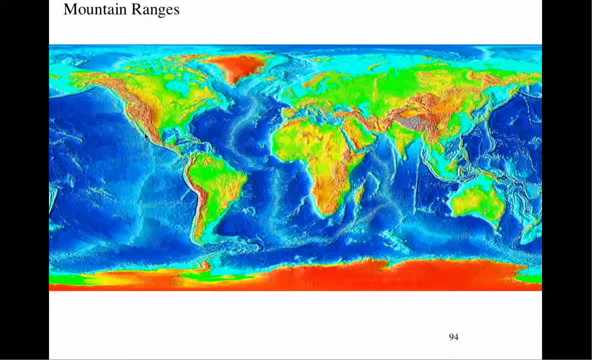 Coastal Range. You have the Coastal Range and the Cascades in here. These, if I'm looking right, are the Sierra Nevadas- Hard to tell. And then back here, although it doesn't look like it, these are mountains. These are extremely old, folded mountains. the Appalachians Again. 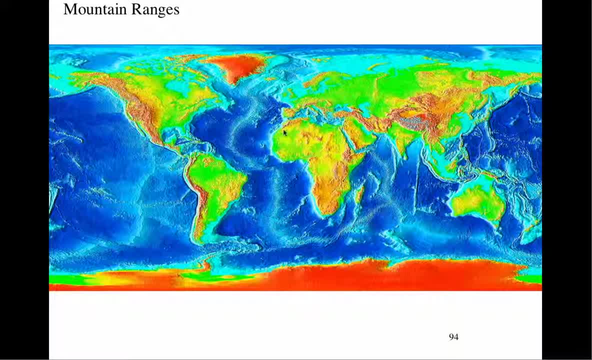 these are the Andes. The Atlas Mountains are right across here where Africa is bumping into Europe, And the European component of that Are the Pyrenees and the Alps right across here, And the Caucasus Over here, where the 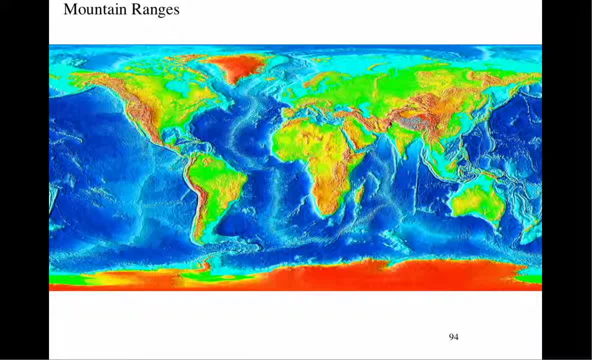 Indian plate is going or banging into the Asian plate. you have the Himalayas And that's it for the major mountain ranges- Oops, I left out the Urals, My bad. And you have the same kind of thing going on over here that you have in Alaska: A lot of accretionary. 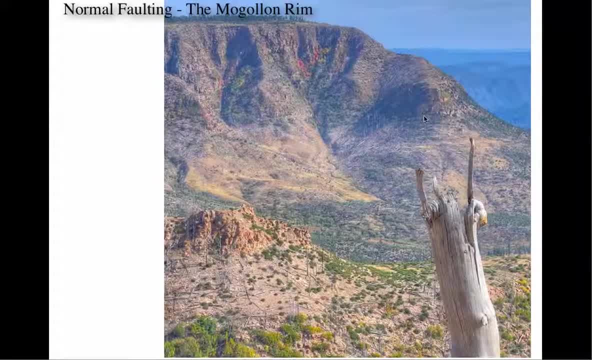 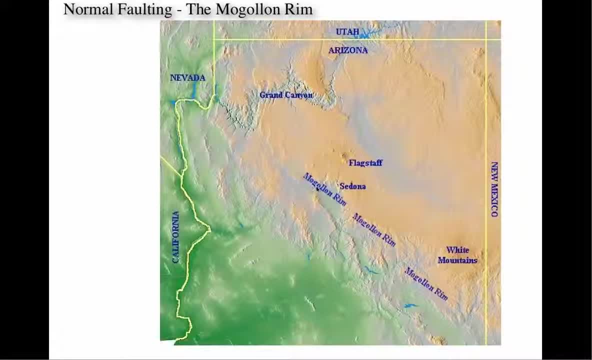 terrains. Okay, normal faulting. In Arizona we have a really big normal fault. It is called the Mogollon Rim and it stretches all here across Arizona. If you ever go up on the way to Winslow, the most important town in Arizona, and pass Pine and Payson, between Pine and Payson. 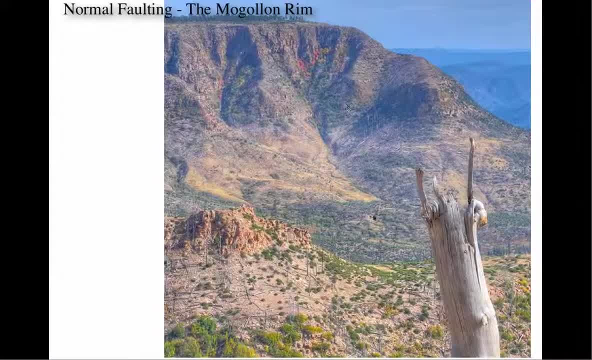 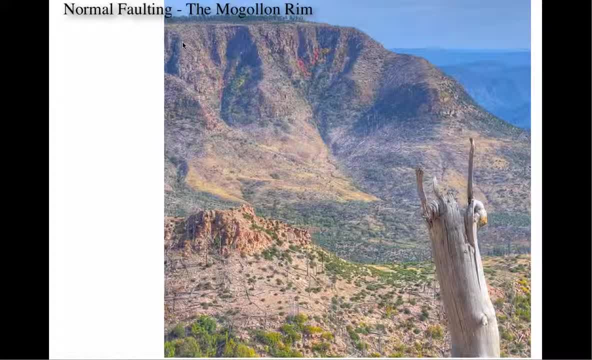 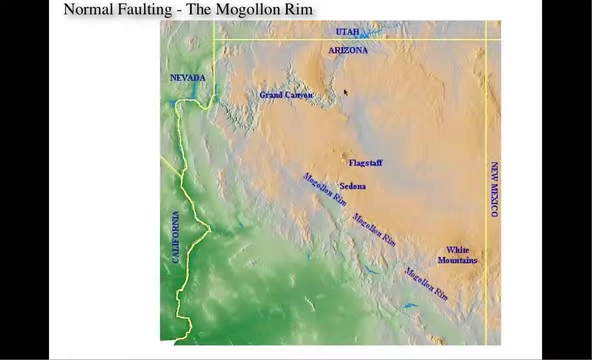 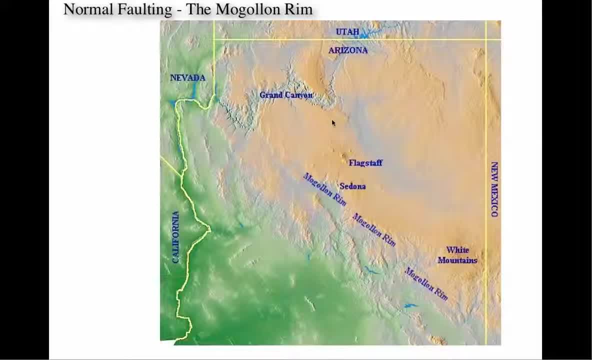 plateau that forms the Grand Canyon, the Kaibab Plateau, and the plateau itself is bisected by the Colorado River. Here's the North Kaibab and the South Kaibab. The North Kaibab is about a thousand feet higher than the South. All right. 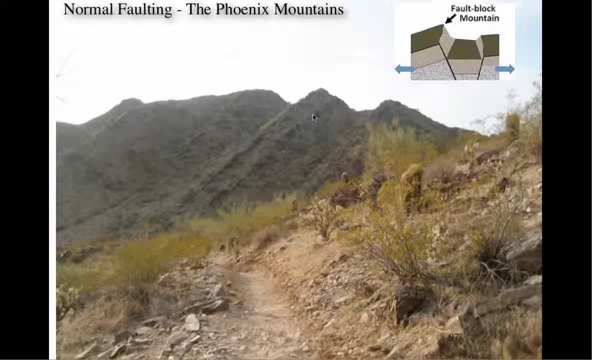 next we have normal faulting in the Phoenix area. Here's a fault block mountain. This is kind of convenient, because this is the same as this, it's just that the real one is tilted more. This is broken and tipped back and you. 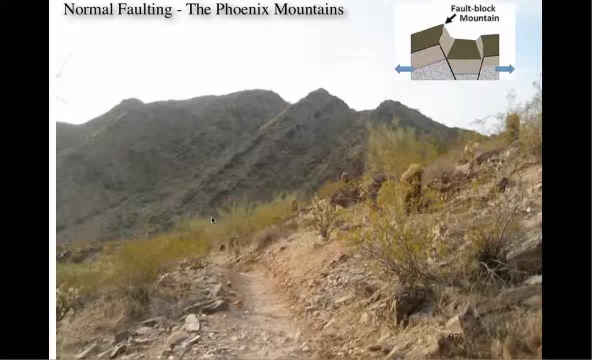 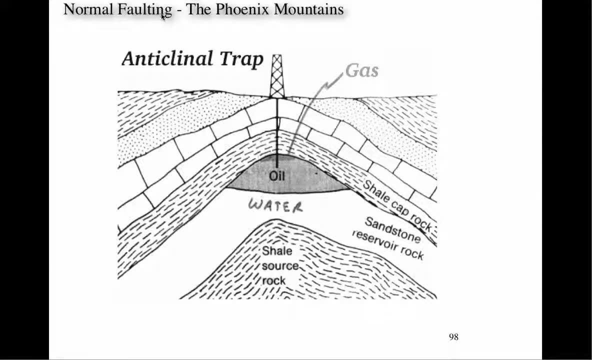 will find this all over in the Phoenix Mountains. This is really kind of cool. Whoops, Let's get rid of that topic. Ignore that. That has nothing to do with this. We've talked about this briefly, but I wanted to clear up a few things. 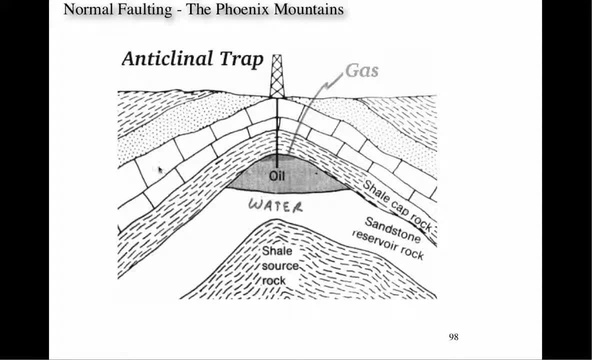 Anticlinal traps form in sedimentary rocks, and you get them when you have a shale rock as a cap. Remember how a shale won't let water down from the top. Well, the same thing happens when oil, water and gas- natural gas- try and rise. 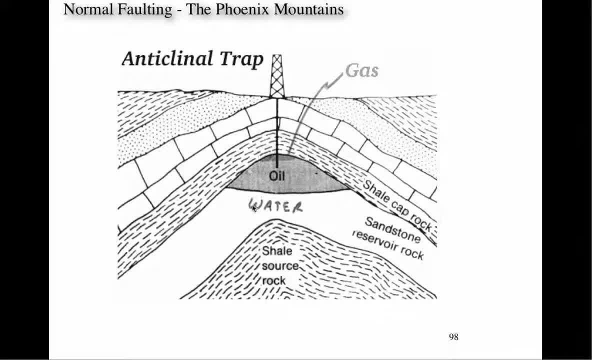 up through the rock. They can't. Now the water is down here. it's trapped. The oil and the gas are less dense than the water, so they go on top The water, or the rock in which the oil, the gas and the water are trapped is sandstone. 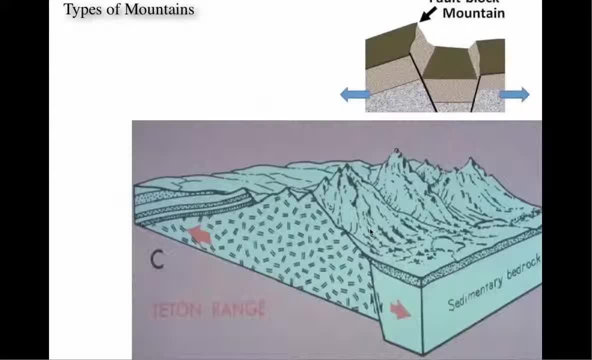 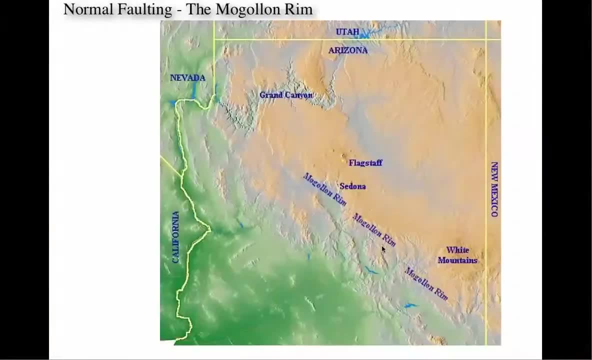 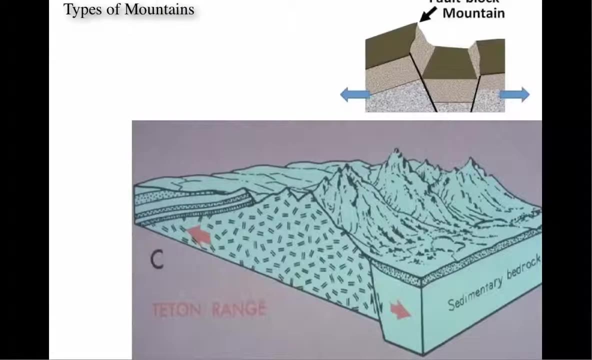 Those are just a few important things I thought I'd point out Again: Fault Block Mountains, The Tetons that I showed you a while ago, The Tetons- This is the edge of the fault block front. This is the edge of the Tetons. 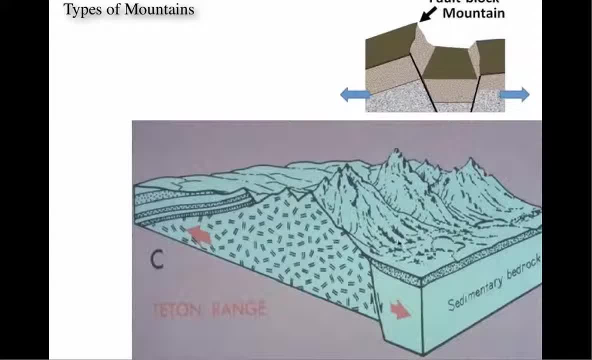 That picture was taken from over here. Here's the little barn. These guys have faulted up and then eroded back, And it's happening because of tension. These pieces of the plate are being pulled on. And why are they being pulled on? Well, over here, the Pacific Plate is going underneath North America. 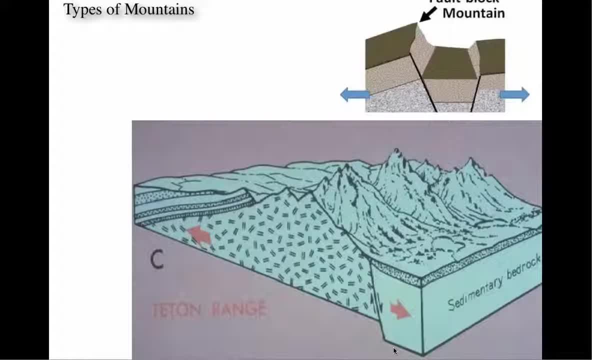 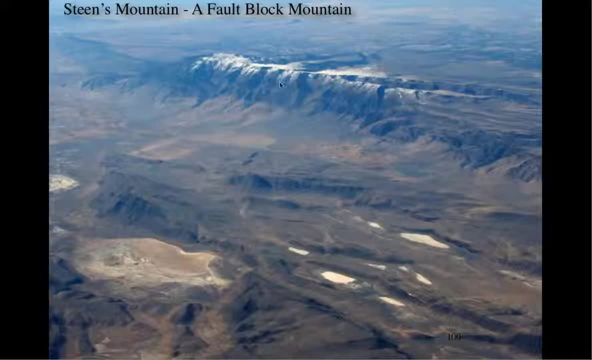 and as it does it stretches out North America because we're resting on top of it. Here's Steens Mountain, another fault block mountain. Here's the fault base. It could have been way out here somewhere, but it is eroded back over. 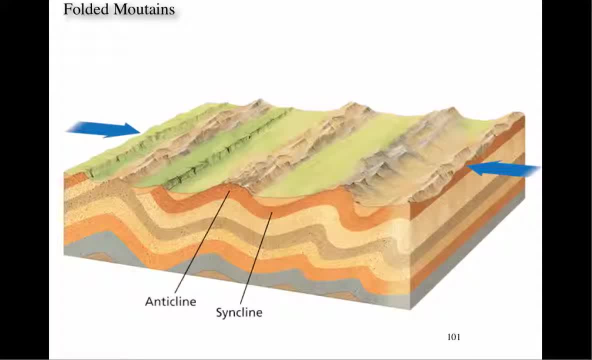 time, Oops, And again. folded mountains, Anticline and a syncline. Now this is kind of weird, because the drawing isn't exactly right. The anticlines most often make the valleys because these rocks are worn down, and the synclines being 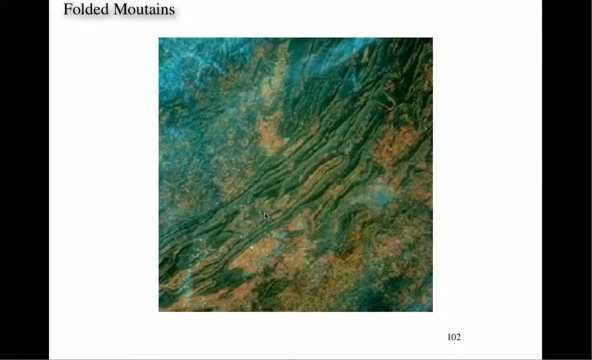 squished together quite often make the hills. Where do you see folded mountains Again? the Appalachian Mountains, back east Tennessee, Kentucky, Pennsylvania, that kind of area. If you put a towel on top of your table and squished it together, you could have squished it down and that would be an anti-climbing mountain. 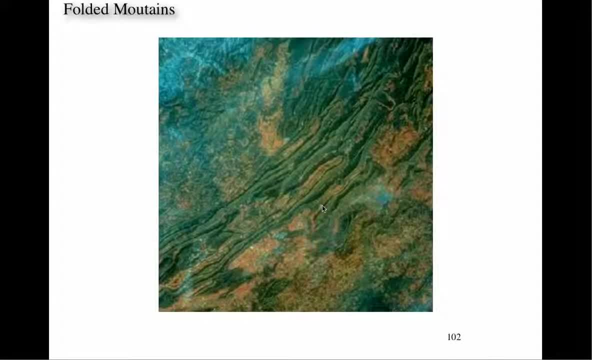 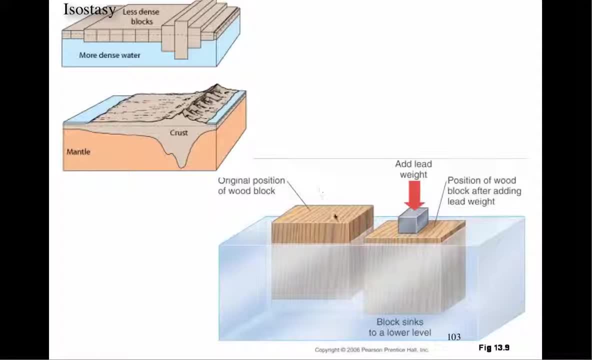 you would get this kind of wrinkling. This is looking down on top of the towel or on top of the landforms back east Now isostasy. This is something people don't think about. Here's a wood block floating in water, If you add some. 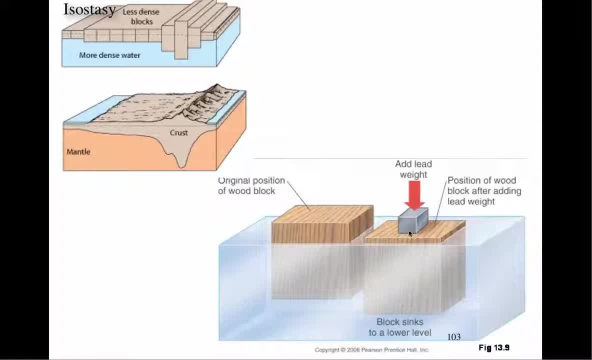 weight on it, the wood block will float a little bit lower. If you take the lead weight off, the block will float a little higher. Well, the crust of the earth is the same way we are floating in the mantle, And if some of the stuff is, 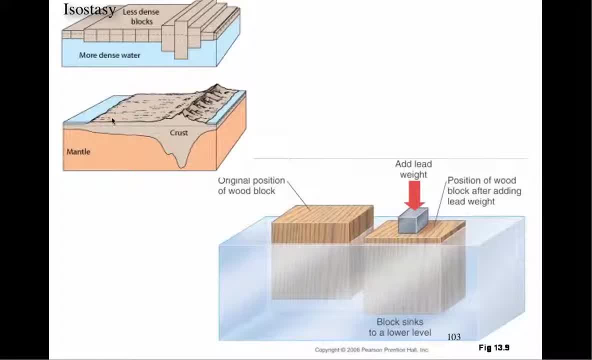 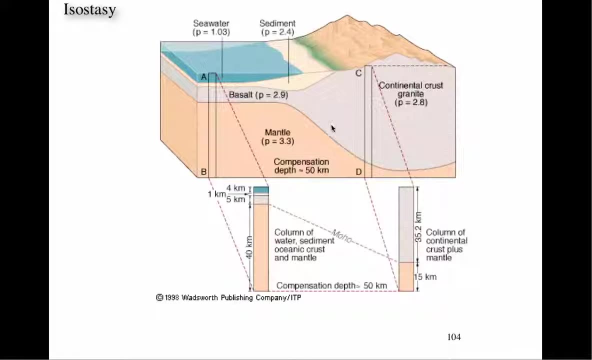 eroded off the top, the crust will bounce back. We're kind of like an iceberg in that most of our stuff is actually below what we would call the waterline or the median line. Every time you see a mountain, it has roots that go. 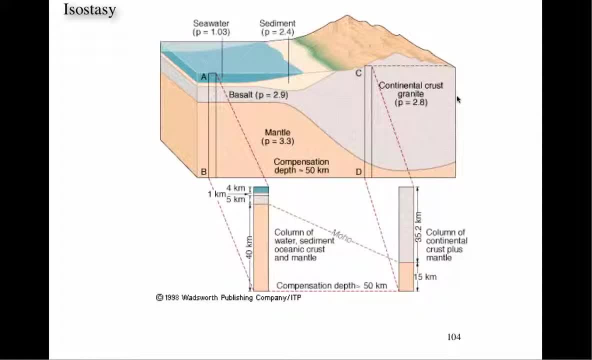 down into the mantle very far. Just something to think about. When the top of the mountain wears down, this bounces up a little, Wears some more off, this bounces up Joints and faults. You know that faults are lines along which there's been. 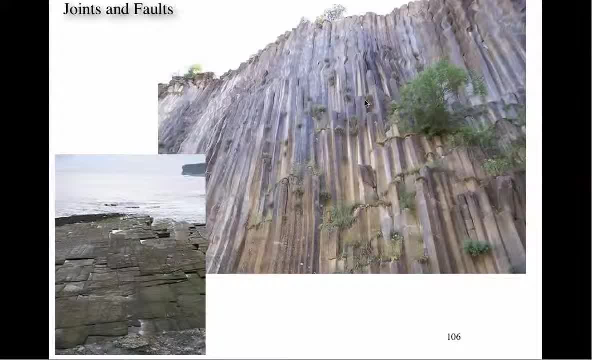 movement, but joints are just cracks in the rock. These are joints in rock. This is in- oh, I want to say Scotland, I'm not sure, But this is just a joint set. where rock is cracked, There's no movement. But this is a great place for water and 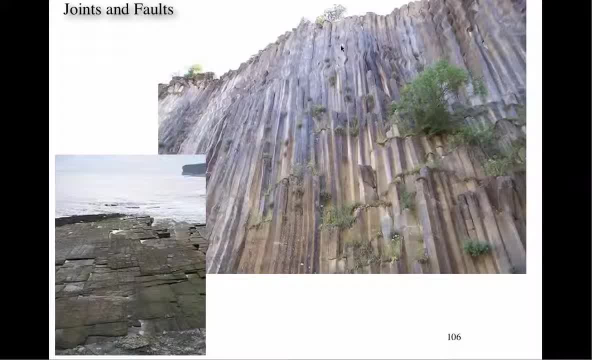 roots to get down in and then they crack apart rock. This looks like Devil's Tower in Wyoming, but it's actually somewhere in the Mideast, I think. And this is a what's called columnar jointing, When basalt comes up through the ground and